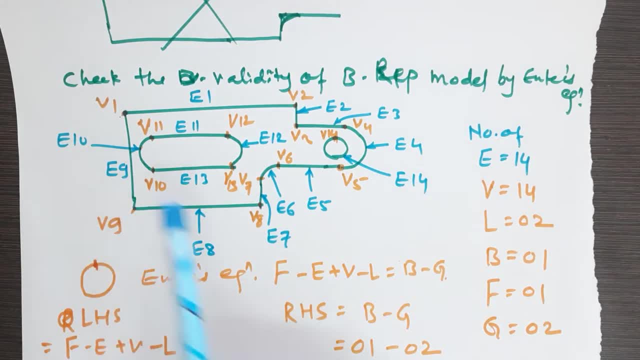 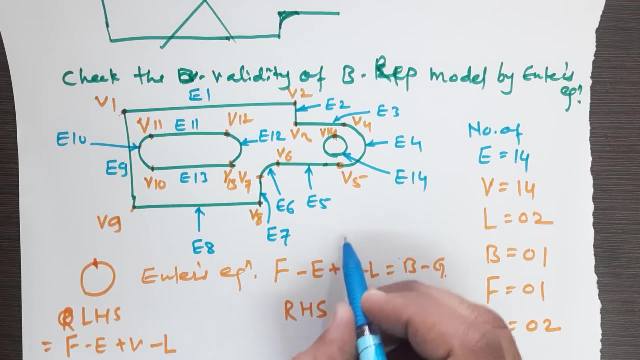 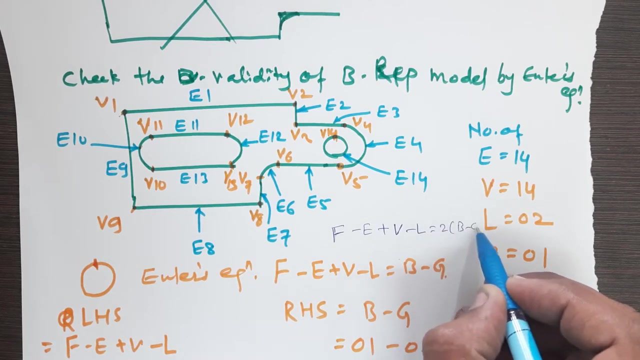 So here, most important thing is you need to remember this equation. Euler's equation is: F minus E plus V minus L is equal to B minus G for 2D. Okay, so this equation will be for 2D geometry. and if suppose 3D geometry will be there, so same equation will be there, like this: F minus E plus V minus L is equal to 2 times B minus G. Okay, so this equation will be for 3D geometry. 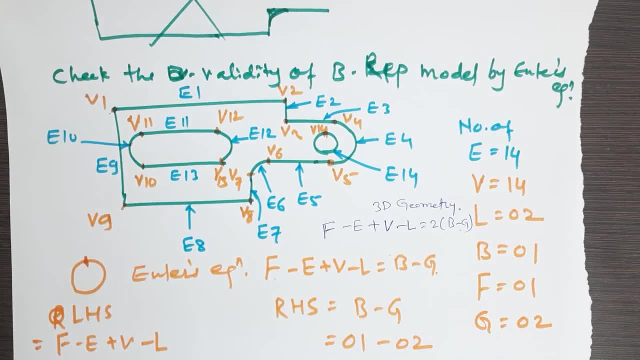 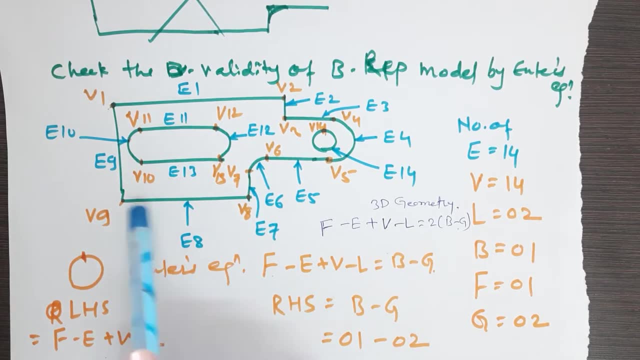 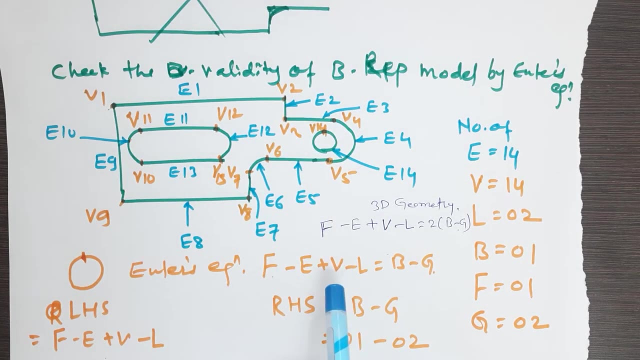 Okay, So here what you need to do is here: F is nothing but faces, number of faces, E is number of edges. number of edges means number of lines. V is number of vertices, means corners. Okay, so everywhere corners will be called, as here, vertices. L is number of loops, Okay, closed loops, Then is equal to. B is nothing but number of bodies, and G is number of genus or number of through holes. Okay, you can remember like this: through hole. 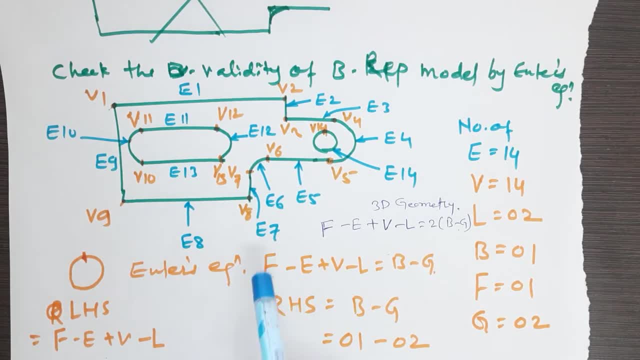 so here, first thing, we need to check the number of faces, edges, vertices, loops, bodies and through holes. so let us start with this number of faces or number of edges anywhere you can find. so here, number of faces in this case- you can see here the total geometry- have only single face. 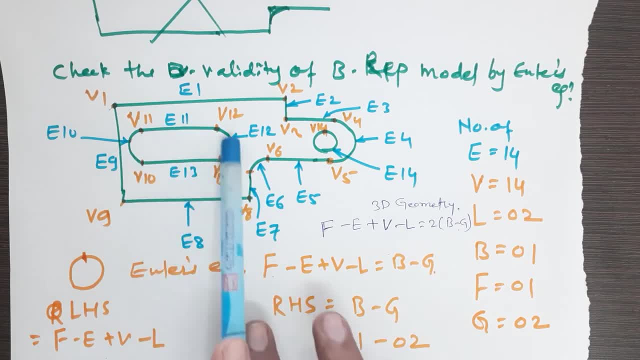 so it is like a paper which is cut like this, and here one hole will be there. so the number of faces will be one only. so F is equal to 1, now number of edges. if we count. so number of lines, you need to count. so, from here to here, one line is there. from here to here, second line, E2. 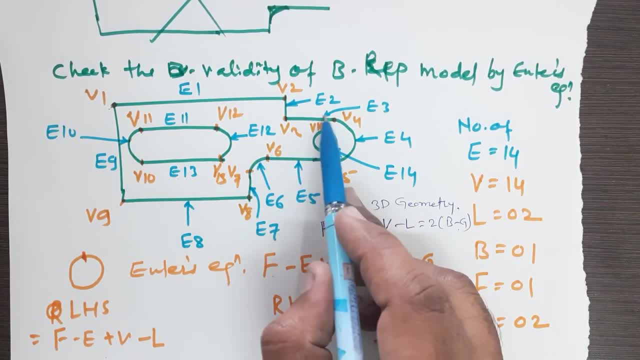 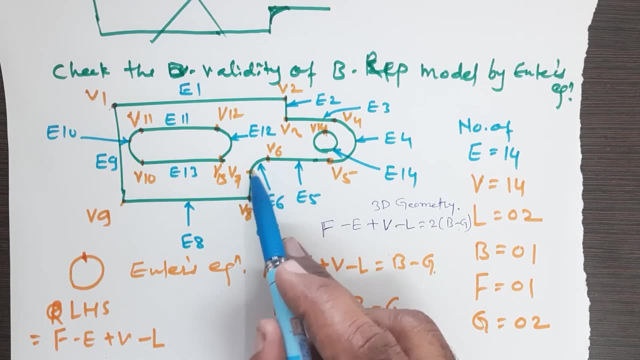 then, from here to here, E3- this arc is E4. then from here to here, E5 and this small arc will be there. E4 and this small arc will be there. E5 and this small arc will be there: E6. this line, E7, this line, E8. this line, E9. 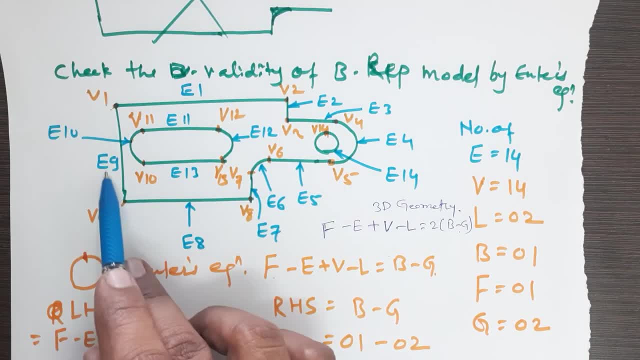 so this outer body is having 9 edges. then we will go inside. so from here to here, this arc is E10. from here to here, E11. from here to here: E12. from here to here: E13. so total 13 edges. then if we see here a circle, is there again. 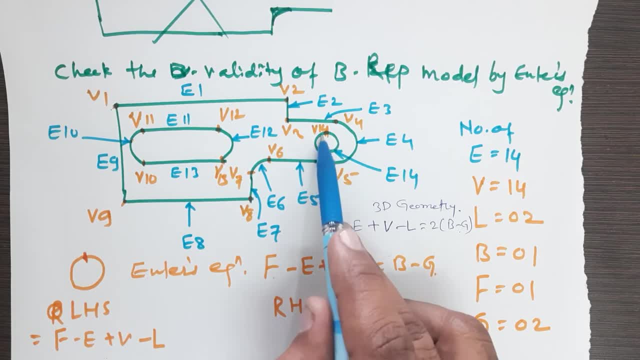 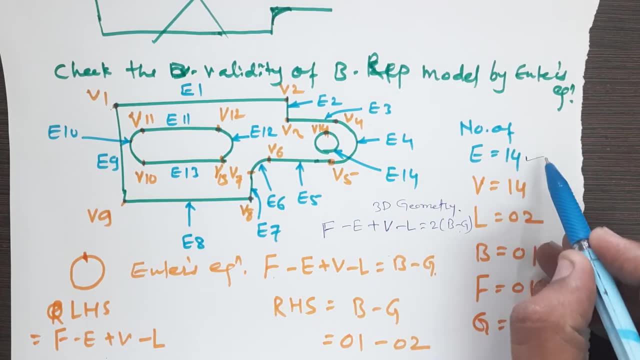 so this circle will have only one edge, so it will start from here and it will end here. so E14. so total number of edges are 14. then after that number of vertices, if we count number of vertices, so let us say we will count here corners. 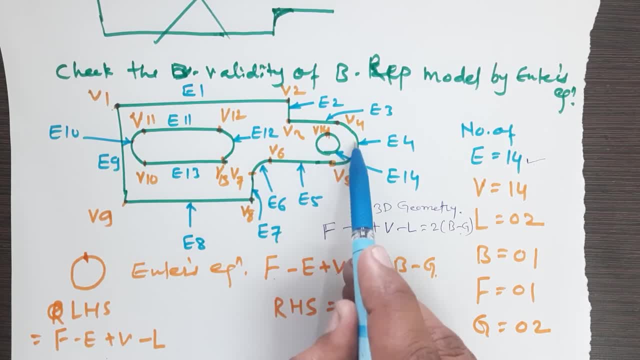 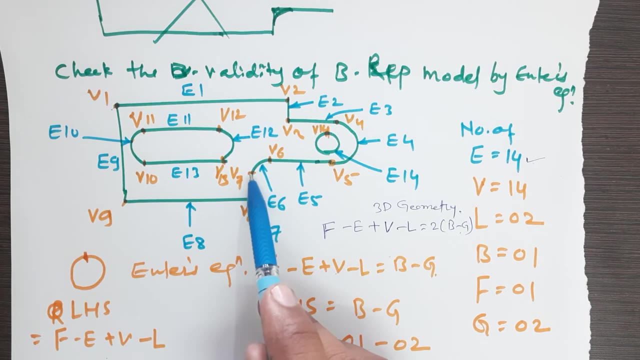 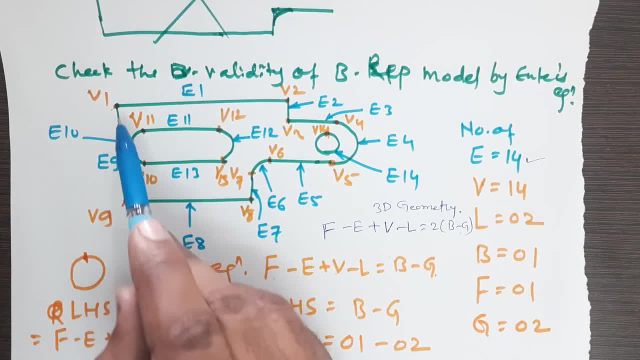 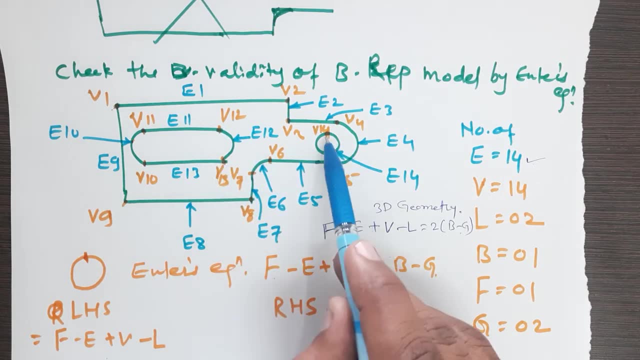 then this corner will be V8, then V9 and if we go inside, V10 will be here, V11, V12, V13, and if we see here one circle is there, so circle is having only one point, okay, so V14. so your number of vertices. 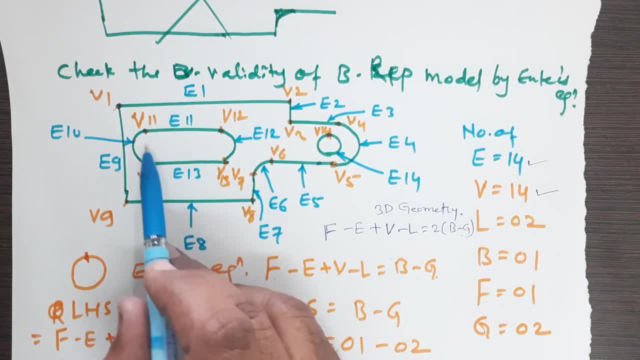 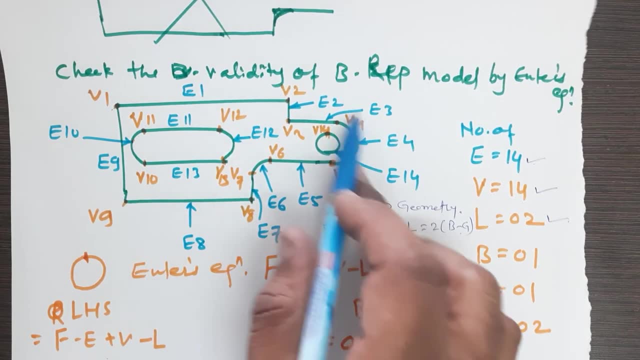 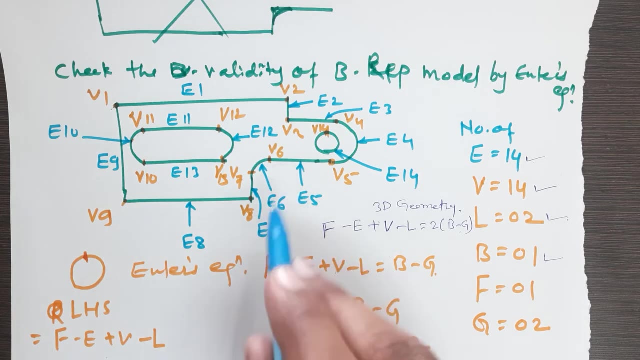 are 14. then number of loops: number of loops are here it is a closed loop and here it is a closed loop, okay, so two loops are there, so number of loops are two. now this complete face is having only one body. okay, in single body. this complete face is we are defining the number of, is we have. 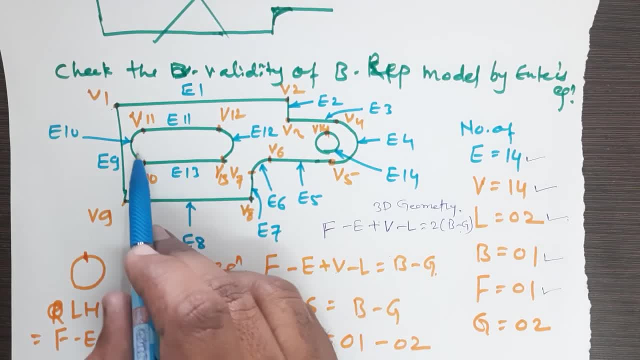 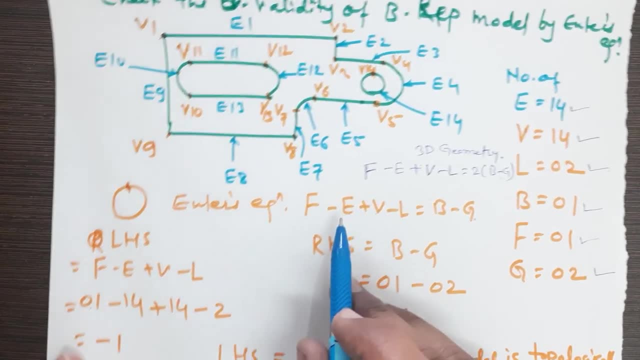 already discussed, it is one, and number of genus means number of through holes. so here this is through hole and this is through hole, so two through holes are there. okay, now we will check here this validity, this equation. okay, so we will see first left hand side and then we will go for. 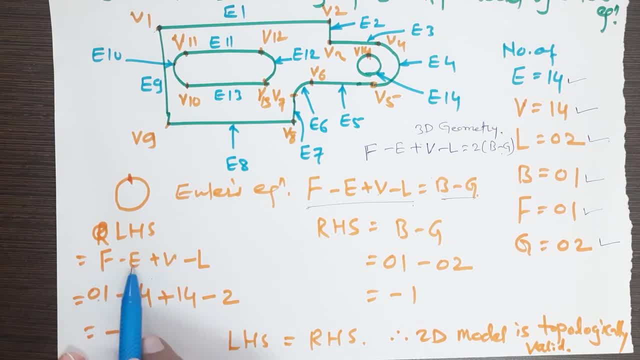 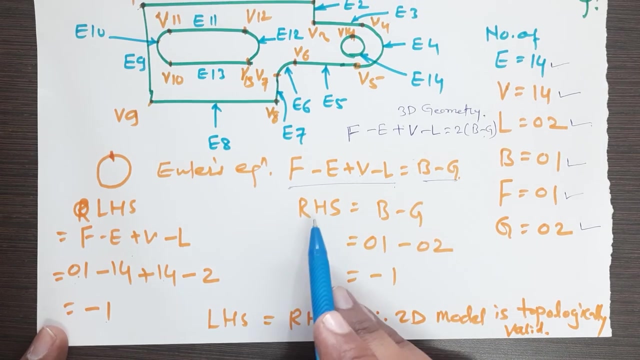 the right hand side. okay, so left hand side, LHS is F. okay, so left hand side, LHS is F minus E plus V minus L. F is 1 minus 14, plus 14 and minus 2. okay, so we are just substituting these values of F, E, V. L is equal to minus 1. now we will see right hand side, so B minus G is there. 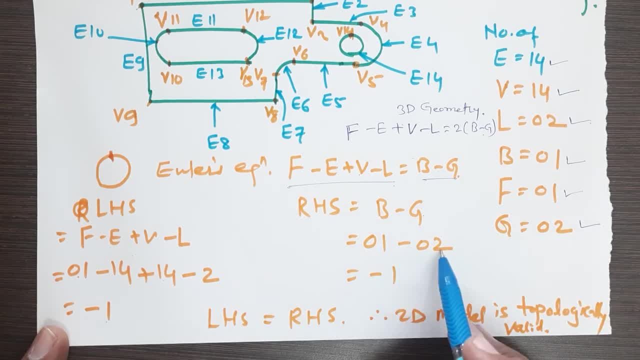 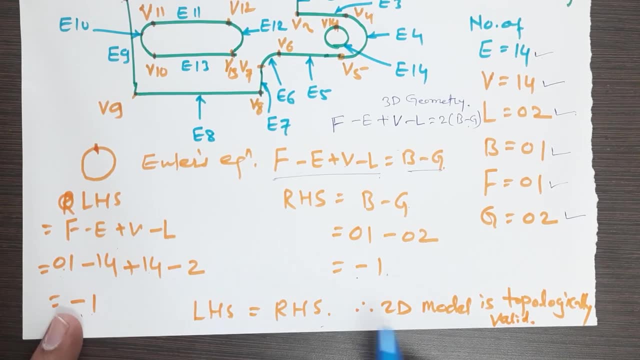 so B is 1, G is minus, G is 2. so 1 minus 2 will be minus 1. now, here minus 1, here minus 1. LHS and RHS: both are equal, both are same. hence this 2D model is topological valid. okay, so in this.